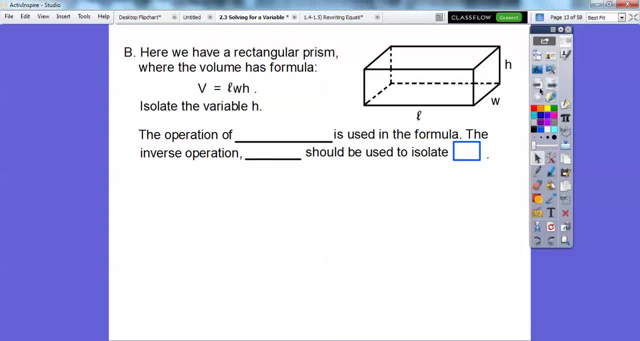 we have a rectangular prism with the volume formula. Okay, so the volume formula is: volume equals length times width, times height. right here, So let's isolate h, right here. Okay so the operation of when we see l, w, h, that means multiplication, So the operation of multiplication. 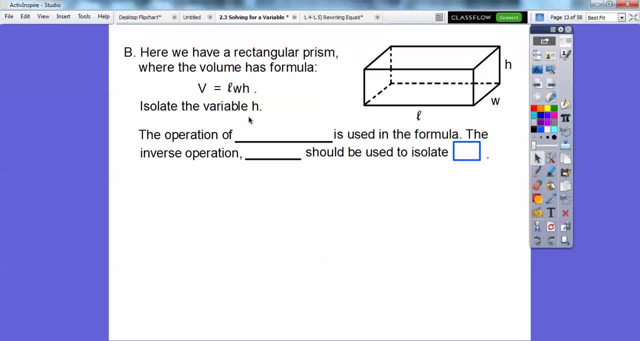 is used, And so the inverse operation is division. It should be used to isolate h, right there, Okay? so let's go ahead and do that. Let's divide both sides by well. the things that are being multiplied with h are these l w. So let's divide both sides by l w, Okay, and then? 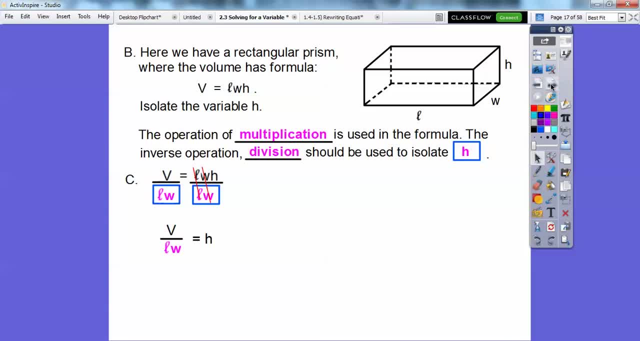 the l's will cancel, the w's will cancel. So there's our h formula: h equals v over l, w, And that's your answer, right there. Okay, when it says solve for h, right there? So this formula, rearranged in this way, could now easily produce the height of a rectangular. 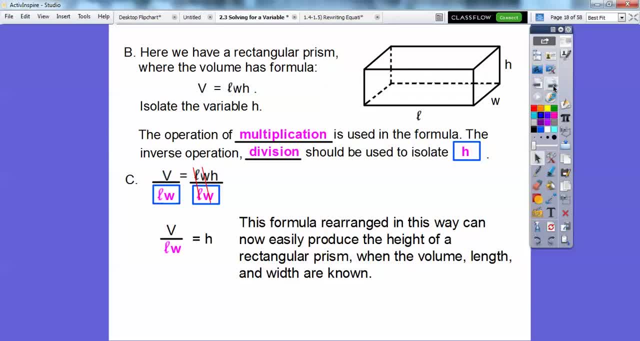 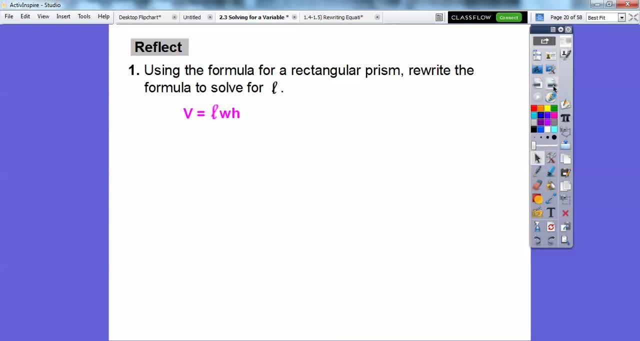 prism when they give you the volume and the length and the width. Okay, so we'll do some of that. So, using the formula for a rectangular prism, rewrite the formula to solve for l. Okay, so let's go back to volume. equals l w h. All right, this time we're going to divide both sides by w, h And then that. 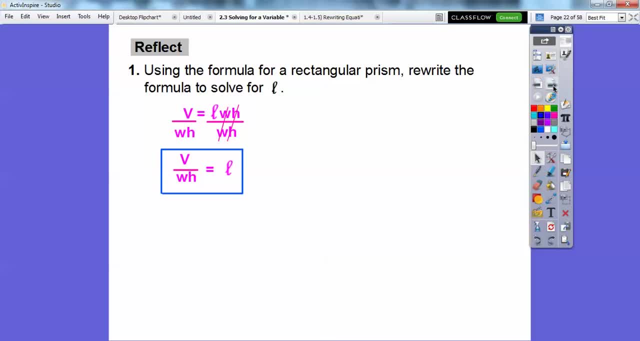 way we get l all by itself. So the formula for this one is: v over w, h equals l. Okay, so this means multiplication, Tongue twister. So we do the inverse, which we divide. So we divide by the things we want to get. 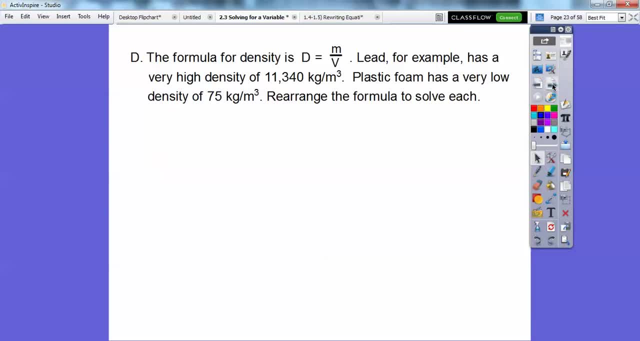 rid of that's tagged with the l, right there. Okay, all right, we'll get used to it. So here's one. The formula density is: d equals m over v, m represents mass and this represents volume, right here, Okay. so lead, for example, has a very high density: of 11,340 kilograms per m cubed, I think. it's mass cubed, And plastic foam, for example, has a very high density of 11,340 kilograms per m cubed. Foam has a very low density: 75 kilograms per meters cubed. Okay, so rearrange the formulas to. 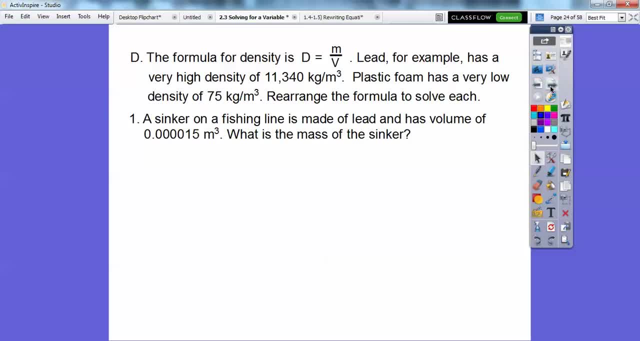 solve for each. Okay, all right. so here's number one. A sinker on a fishing line is made of lead and has a volume of- okay, I'm not going to say that- Actually ten hundred thousandths, ten thousandths, hundred thousandths, millionths, 15 millionths, meters cubed, Okay, mass cubed. So 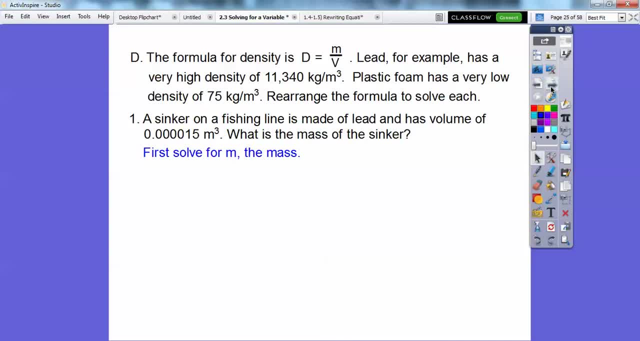 what is the mass of the sinker right there? Okay, so we're going to first solve this formula up here for m to get the mass right here. Okay, so there's our formula, and then we're going to multiply both sides by v to get the v's to cancel. 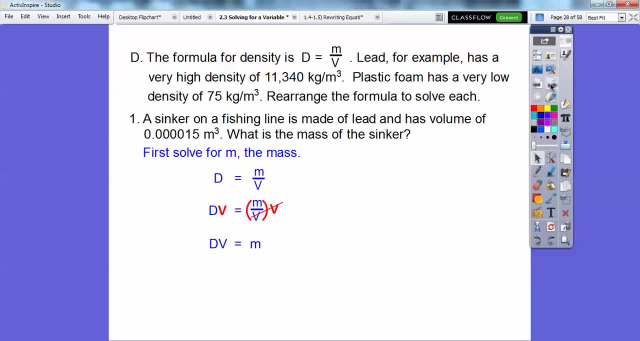 right here. So we get dv equals m. Okay, well, now it's all solved for m. So now all we got to do is plug in the density and the volume- The density they gave us right here and the volume they gave us right here. So we're just going to plug that in right there and we're going to pick up our 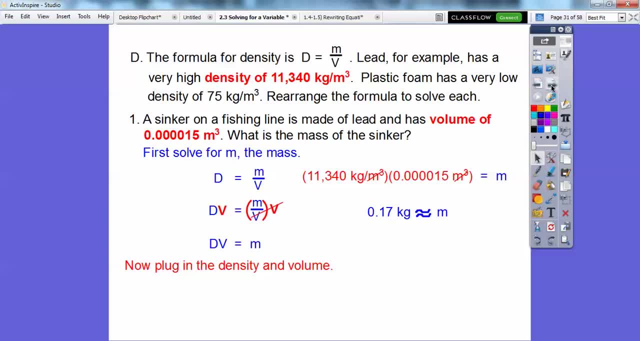 calculators and when we multiply that we get about 0.17 kilograms right here. Notice the mass cubed on the denominator right here cancels out with this mass cubed. that's not in the denominator, in the numerator right here. Okay, all right, let's try another one here. you guys So same. 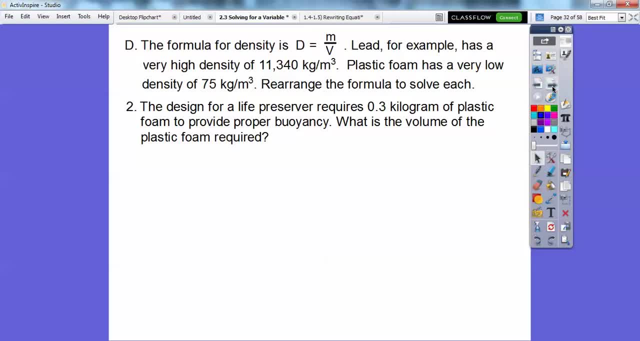 stuff right there. So to design, or the design for a life preserver, requires 0.3 kilograms of plastic foam to provide proper volume. So we're going to plug that in right here and we're going to see what is the volume of the plastic foam. Okay, now we're going to take this equation and solve. 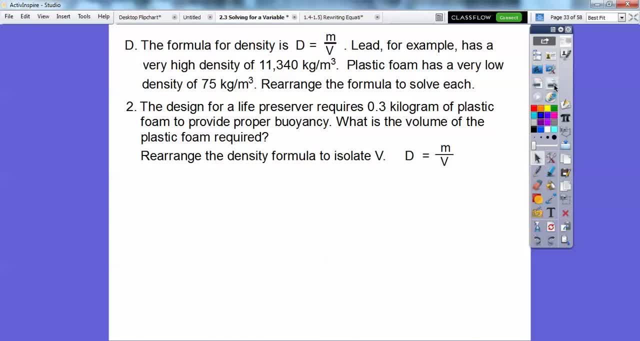 for v, So let's solve for v. Okay, all right. so since v is in the denominator, we don't want it in the denominator, We want it upstairs. So let's multiply both sides of the equation by v. Okay, 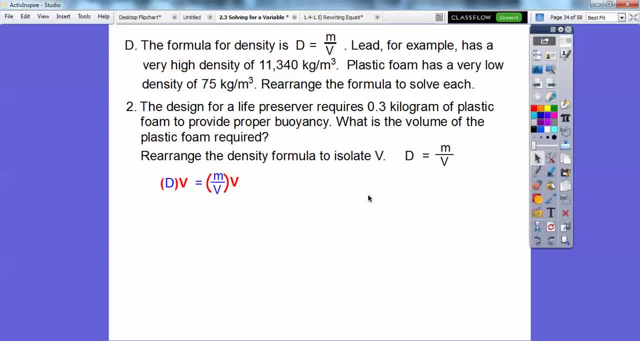 so then, now these v's are going to cancel right here, and then we're going to have dv equals m. Now, remember, we're solving for v, So we got to get rid of this d, right here. Well, this means that we're going to do the inverse, which is divide. Divide both sides by d, right there, and 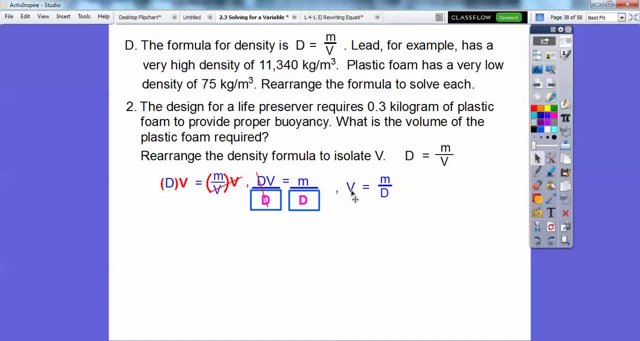 the d's will cancel. So there's our formula isolating v. all by itself, v equals m over d. Okay, so now we just substitute in the given values. Okay, so the density of the foam is here, and then this is the volume right, or the mass right here. So we're going to go ahead and plug. 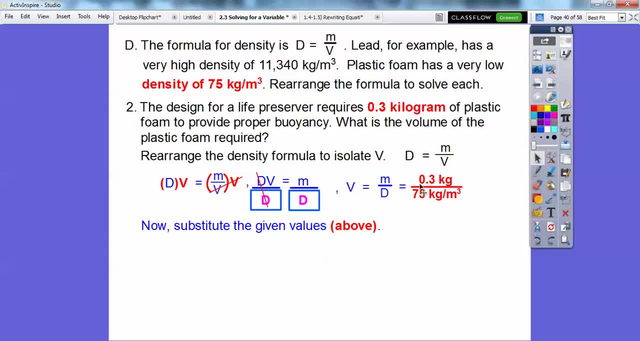 that in right there. So the 0.3 goes right here and the 75 goes right there. Now notice we have a denominator m cubed in the denominator. When that happens, if a denominator is in the denominator, it flips up and becomes part of the numerator. The kilograms are going. 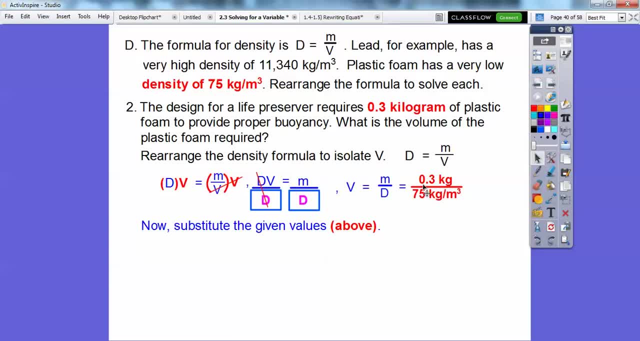 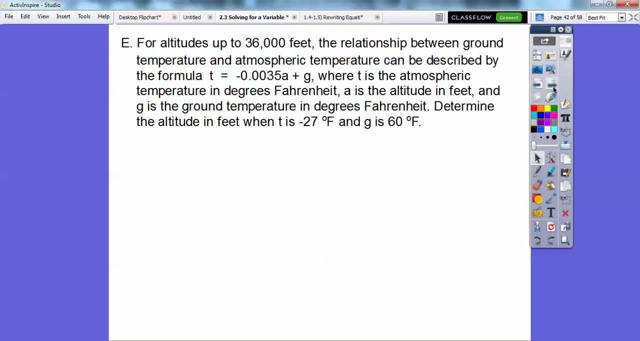 to cancel, because kilogram over kilogram, right there, and then punch it in your calculator: 0.3 divided by 75, right there, We get about 0.004 m cubed right there. Okay, all right, you guys. for altitudes up to 36,000 feet, the relationship between ground temperature and 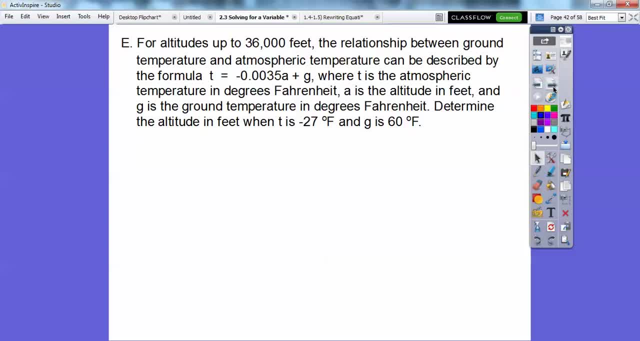 atmospheric temperature can be described by the formula: t equals negative 0.0035a plus g, where t is the atmospheric temperature in degrees Fahrenheit, a is the altitude in feet and g is the ground temperature in degrees Fahrenheit. So determine: here's the big. 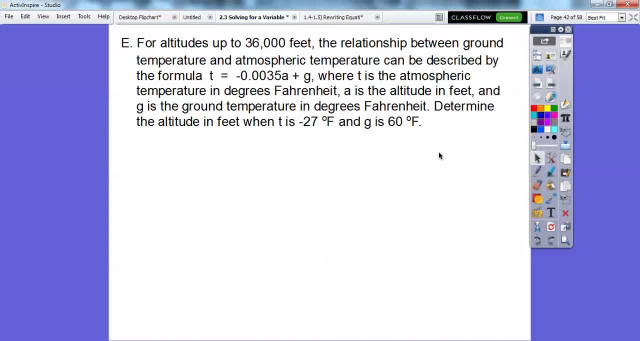 question right here: determine the altitude in feet when t is negative 27 degrees Fahrenheit and g is 60 degrees Fahrenheit. Okay, hasn't that sound fun? okay, well, let's look at this right here. so it says: determine the altitude and feet. so we: 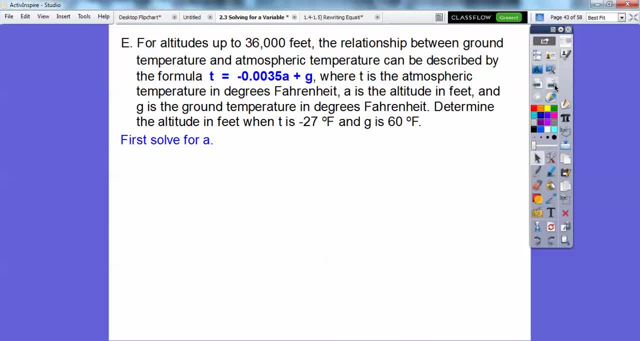 need to solve this equation for a first. okay, so here I'm going to go. what I'm going to do is go minus g on this side and go minus g on this side right here. so do you see that little jump right there? I didn't write it right there, okay. and then now we're going to. this is multiply, so we're going. 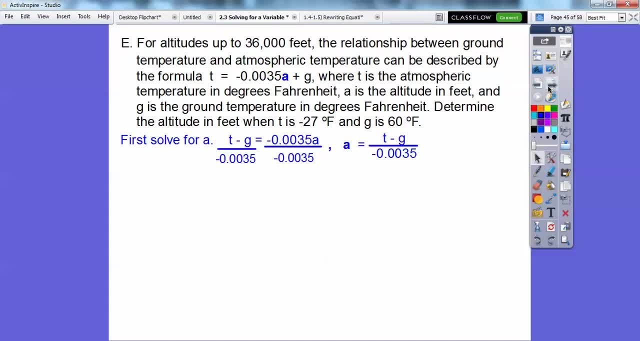 to divide both sides by this decimal right here. when we do that, we get a all by itself, because those cancel right here. a equals the this side over here, okay, all right. so now let's just plug in the values above, right here, okay. so um t. this is t at negative 27 degrees fahrenheit. I forgot. 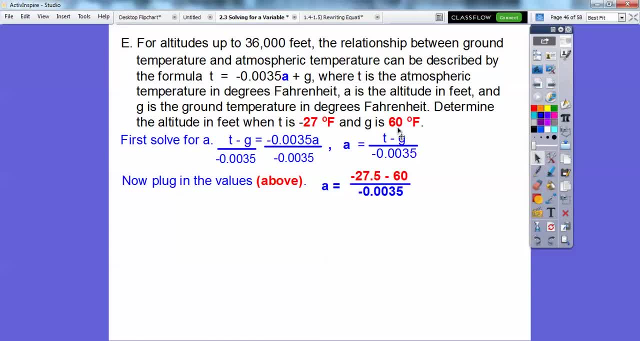 to highlight the negative right there. and then g is 60, so here's t minus g, so it's negative 27.5 minus 60. okay, be careful you guys. negative 27.5 is minus 60 is negative 87.5. okay, when you divide that, you get 25,000. okay, 25,000 feet, okay. so this is determine the altitude. 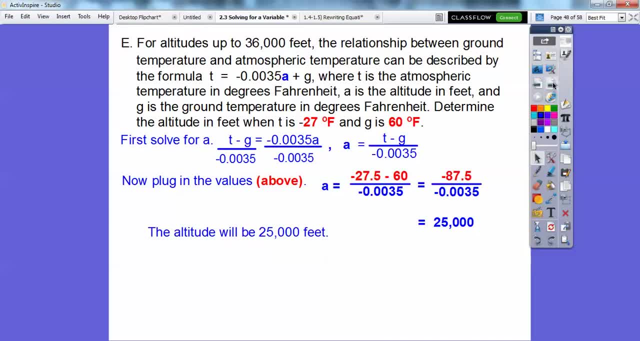 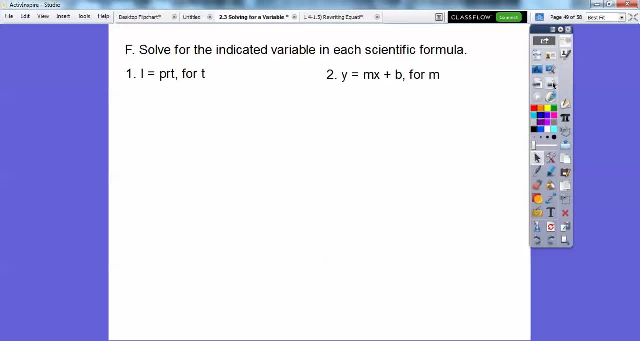 in feet. so the altitude is going to be at 25,000 feet right there. all right, let's try a couple of these. solve the for the indicated variable in each scientific formula. okay, this one's an interest rate at banks and stuff. interest rate equals PRT. that's the principal, that's the rate, that's the.